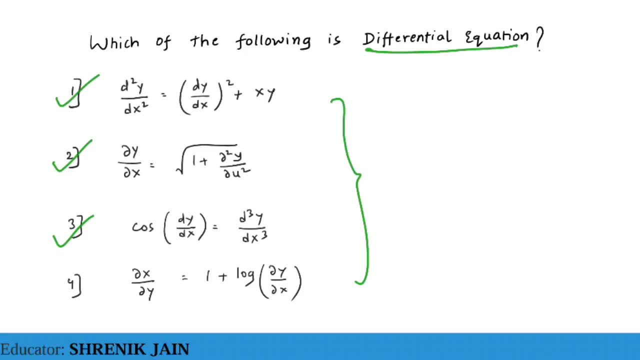 differential equation. then you will say at this point: this is again the two variable and the differential equation, and this is the more than two variable. So partial differential equation. The answer is wrong, because dy by dx, or you can say dou x by dou y or dou v by dou y. They should. 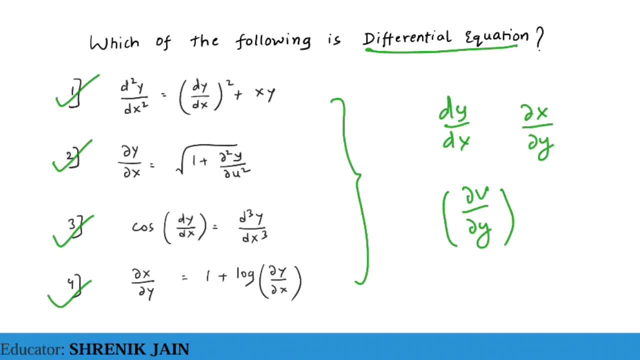 be independent of function. They cannot be treated as the variable. As you can see, here it is treated as the variable cause of something. It cannot be treated as variable. It cannot be treated, okay and also here, as log of something. So these two are not the differential equation, These two 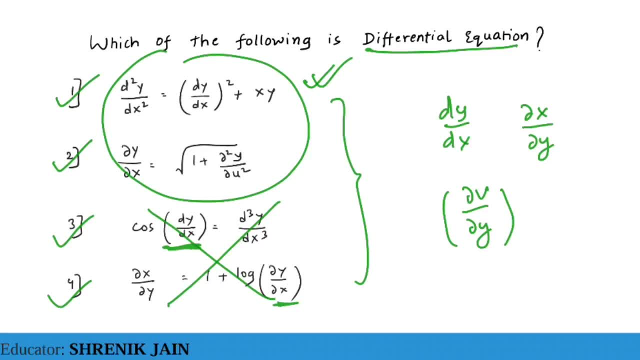 are the differential equation, because here you can see there is no function like cos of something, cos of dy by dx, or dou v by dou u, or sin of something, or log of something, or e raised to of something. okay, So there is no such function in the one and two. that's why these are the 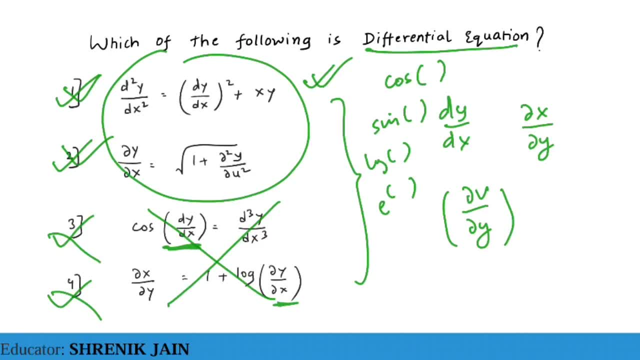 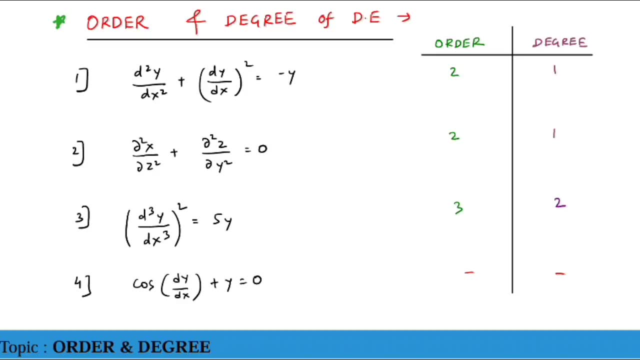 differential equation. and third and fourth are not the differential equation. So now we will study the order and the degree of the differential equation, Very important concept because maximum gate questions are asked on this concept. So what is the order? You have to understand one. 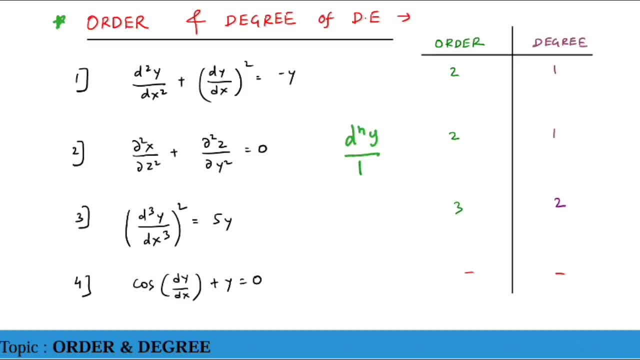 basic thing: d raised to n, y upon dx raised to n, Wherever this n is maximum, okay in the function, in the equation, if n is maximum anywhere. that is the order Now, if you are talking about the power of this function, So this is the power, correct? I am writing the question mark. Power can't be. 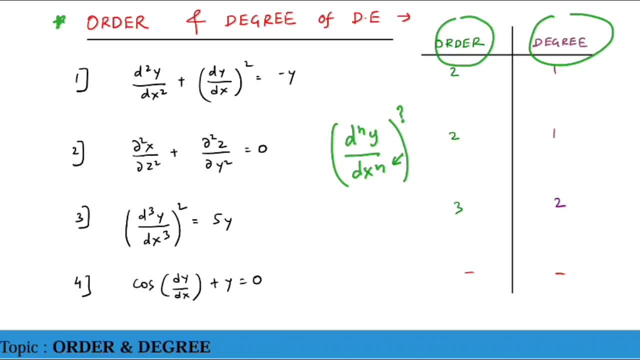 whatever, if you are talking about the power, that is your degree. simple, a very simple concept. So tell me by this equation: if I have d, square y upon dx, square plus dy by dx, the whole square is equal to minus y. what is the order and the degree? to check the order, I will check for the maximum of n. 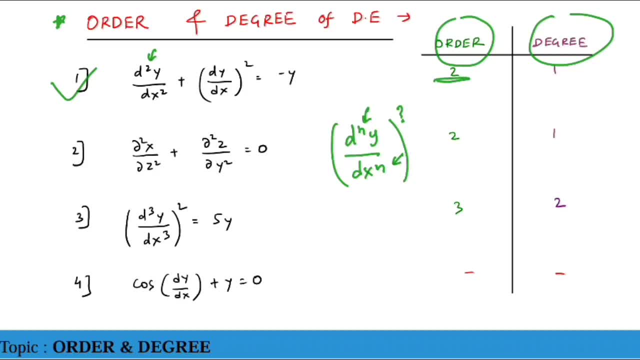 So here n is equal to 2 is maximum. So my order is 2, correct? Now the power of this function is 1.. So my degree is 1, simple. So tell me about the second equation. I have dou square x upon. 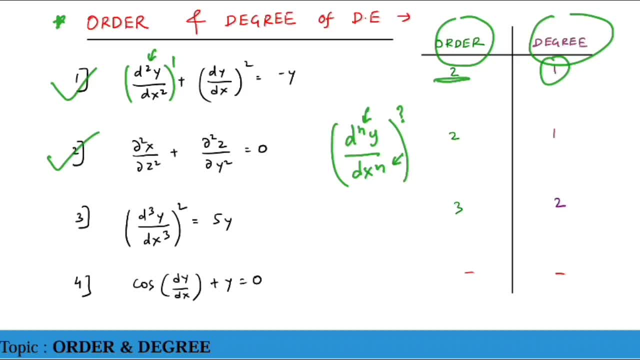 dou z square plus double square, z upon double y square is equal to 0.. Here n is equal to 2.. Here also n is equal to 2.. So n is equal to 2, is maximum is in this equation. So my order is 2.. 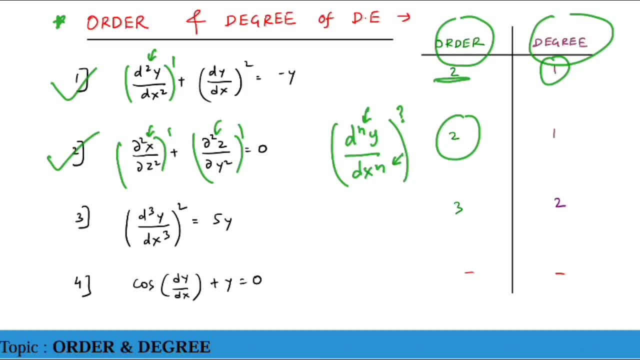 Now, if I take any of this function, my power is 1.. This means that my degree is 1.. So if I take the third example, d cube y upon dx cube, whole raised to 2 is equal to 5y. what is? 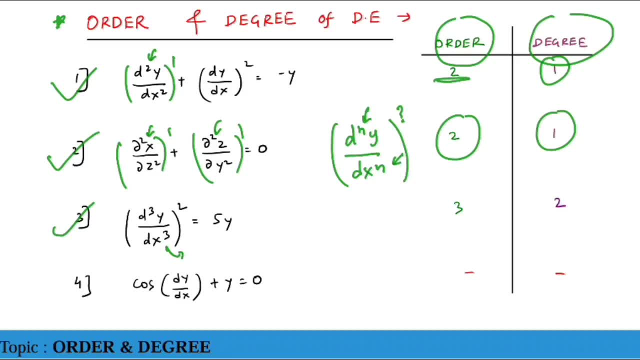 order and degree. Here n is equal to 3, is maximum, So my order is 3 and the power is 2, so my degree is 2. and the fourth example: you cannot consider this as the differential equation, so we cannot find the order and degree because it is not the differential equation. 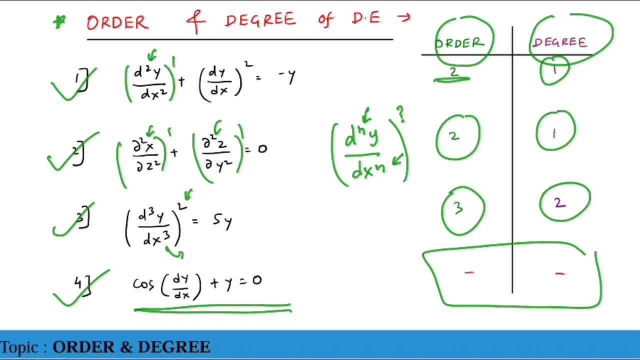 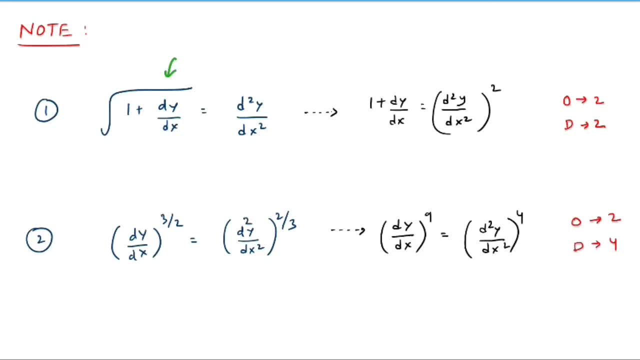 so these are the four varieties of cases, but i want to give you one note which is very important. so this is the note where you can see this power. okay, the power of this equation is something raised to 1 by 2.. whenever you see this fraction part, whenever you see the fraction part, you have to. 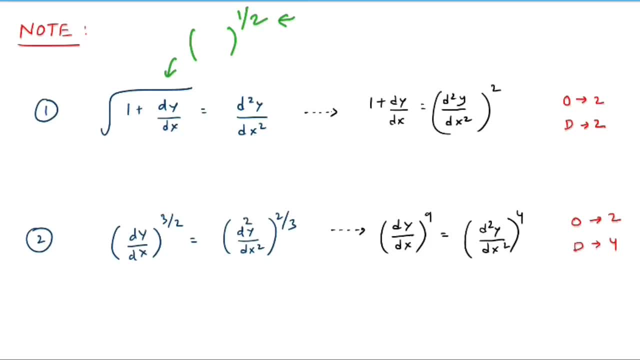 take care that you eliminate this fraction. how you can eliminate this fraction: take square on both the side. if you make it square on both the side, this would be squared and this would be squared, so squared, and 1 by 2 get cancelled, so you will get 1 plus dy by dx, and this term would be. 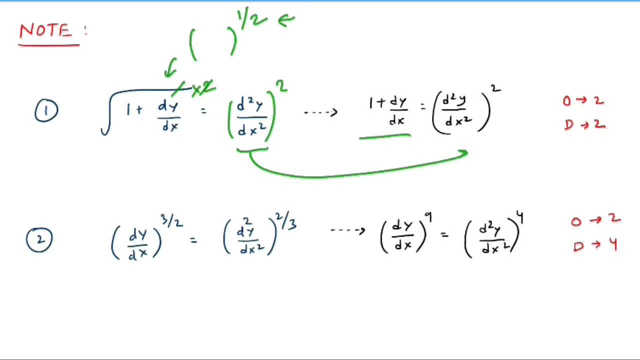 this. okay, now you have to comment on the order and the degree. you can comment only on the order and degree. if you are making this equation free from the radical, that means you are making free from the fraction part. okay, now you can comment. now this is our. 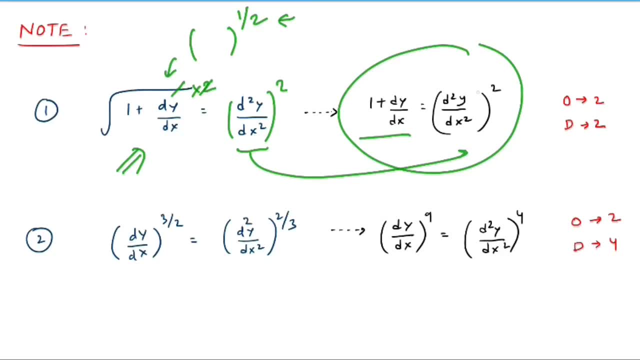 equation, which is perfectly fine, free from the radicals. so the highest power of n is our order. so, as you can see, 2, 2 is our order. and check, check the degree of this function. so the degree is 2, so power is 2, so degree is 2, simple. so this is the second example where square root is not present. 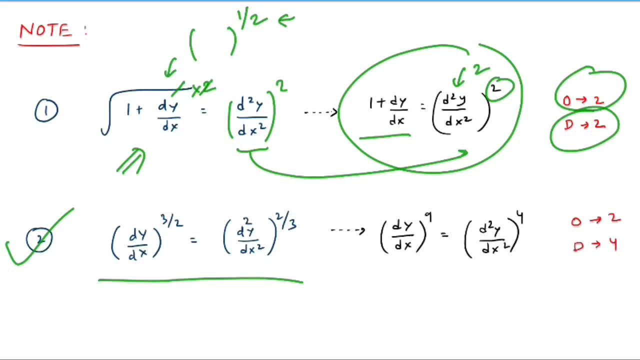 but some different fraction is present, as you can see. dy by dx, the whole is to 3 by 2 is equal to d square. y by dx square, the whole is to 2 by 3.. again we have the problem, we have the radical, we. 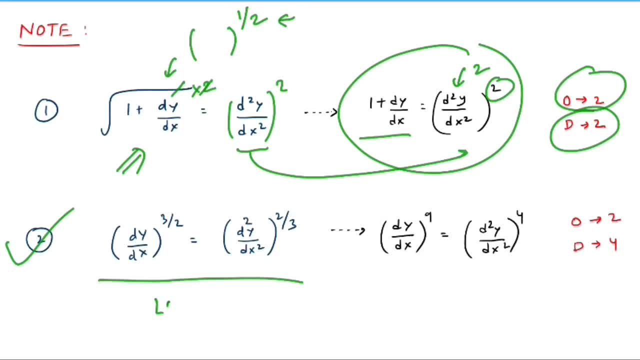 can take this radical. how we can do that? we can take the lcm. take the lcm of 3 comma 2, so it is equal to 6. i will make sure that i am multiplying raised to 6 on both the side. if i do that, i will. 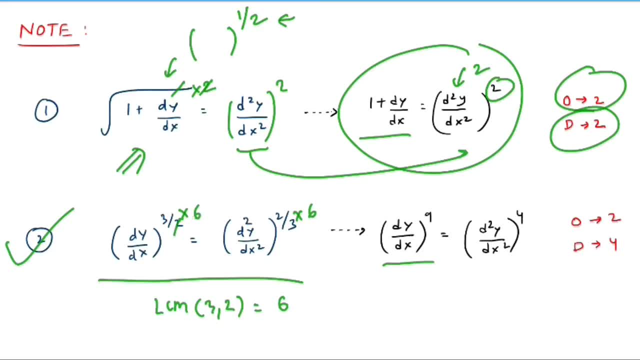 get this, dy by dx, the whole raised to 9, how two, threes are six, so three into three, nine. similarly, three ones are three, twos are two into two, four, as you can see now. now you have, uh, the equation which is free from the radical. now you can comment on the order and degree. so check for the maximum of. 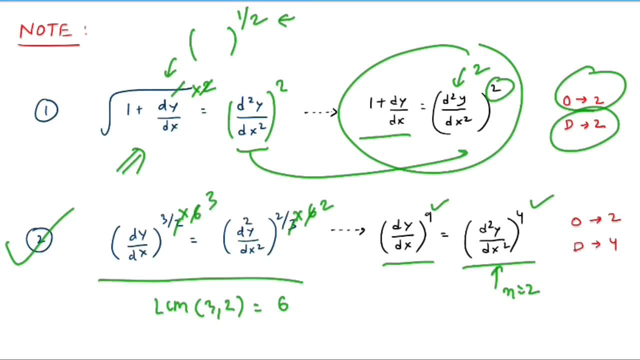 n is maximum here, n is equal to 2. if n is maximum here, this is our order. if i talk about the degree, this means we have to check the power of this function. so power is 4, so decrease 4.. simple, i hope you got all the variations. you know which is differential equation, which is not the differential. 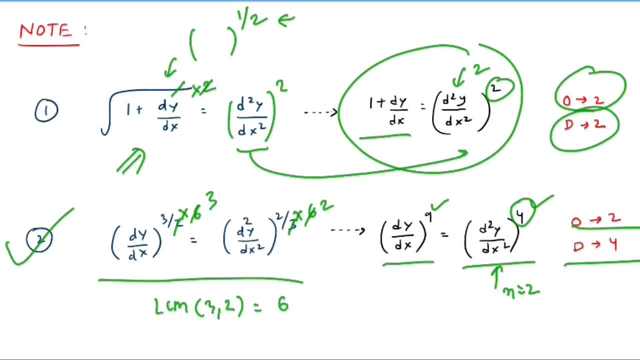 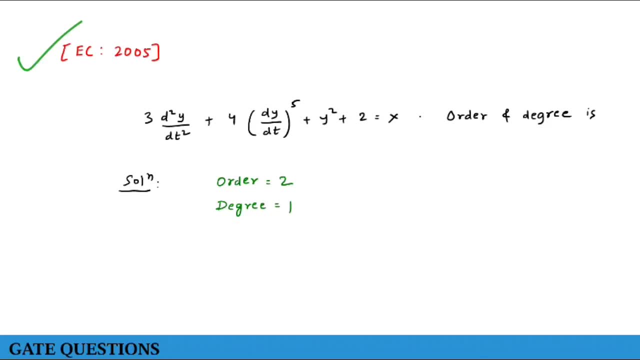 equation, how to get the order and the degree and also how to make sure that our equation is free from radicals. so now we will solve the gate question. so this is telecom 2005 gate question. so this is telecom 2009 question. pretty simple question. again, we have d square y upon d t square. 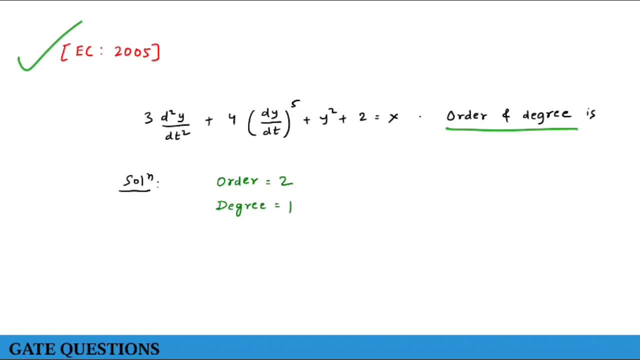 plus 4 dy by dt, the whole power, 5 plus y square plus 2, is equal to x. order and the degree of this differential equation is what? simple, first, to find the order. check for the maximum of n. so n is maximum here. so n is equal to 2 is our order. next, check for the degree. degree means this is our. 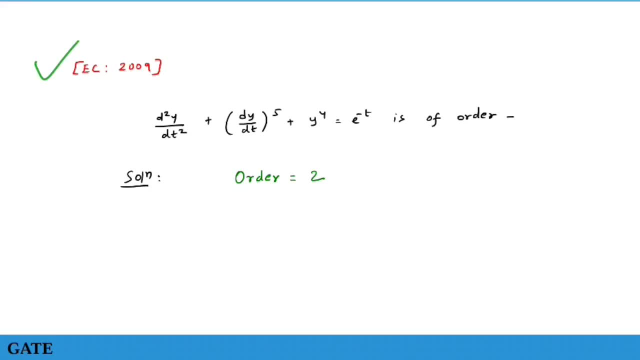 function check for the power. power is 1, so degree is 1, simple. let's move forward to the next question: d square, y upon d, t square. so basically these equations are in y and t and this is the perfect differential equation, or you can say the ordinary differential equation, because they are using the d. 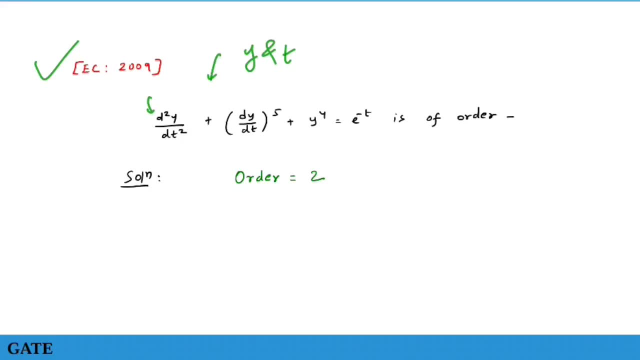 so d square y upon dt, square plus dy by dt, the whole power, 5 plus y. raise to 4 is equal to e, raise to minus t. so what is the order of this differential equation they are asking about? the order? order means maximum of n correct and degree means you have to check the check the power. so they: 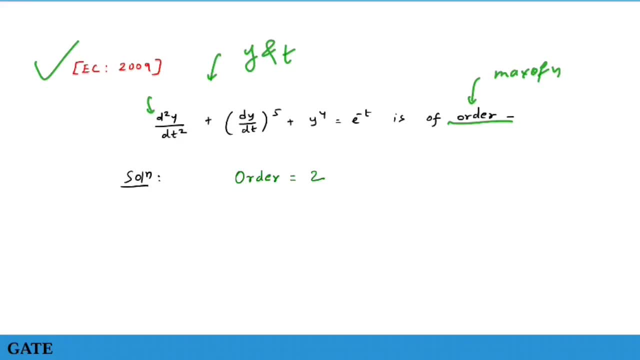 are asking about the degree, so you have to make sure you are finding only the order. so order is: is what? n is equal to 2 here. n is equal to 1 here. so n is equal to 2 is maximum. so order is 2 simple. 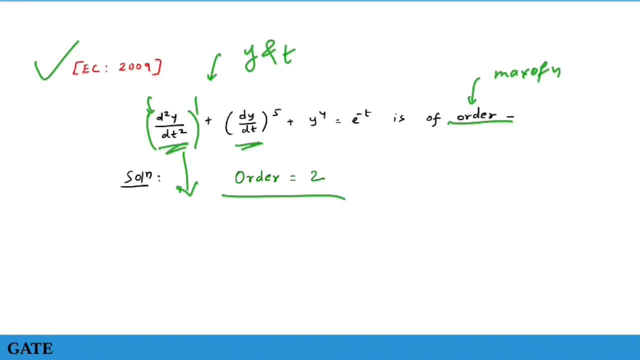 if they told you to find the degree, what you have to do check the power. so power is 1. so, uh, degree is degree would be: what degree is 1.. so i hope you got the basic idea. now i want you to comment the answer about this question. of this question is computer engineering 2007 gate question. 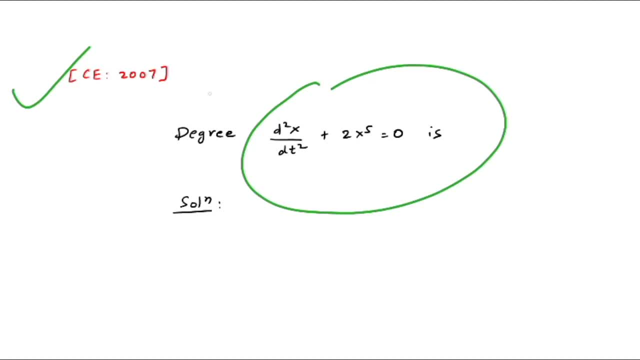 degree of this equation is what? so degree, or you can say the power are same. okay, this was the question, but i also want you to comment on the order. so what would be the order and what would be the degree of this differential equation? so make sure you comment. i will tell you whether. 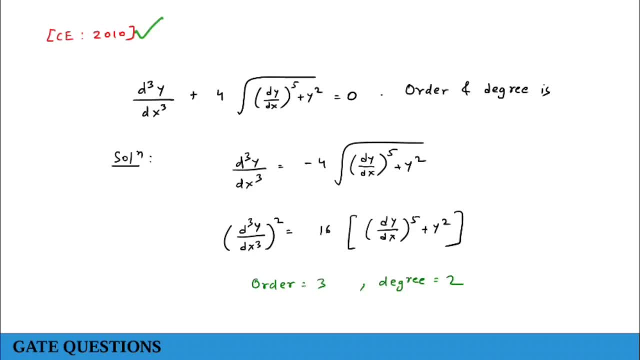 it's right or wrong. now this is computer engineering 2010 gate question. very interesting question d to the power 3y upon dx cube plus 4 root of dy by dx, the whole power 5 plus y square. find the order and the degree of this differential equation. so most of the student will go for this. 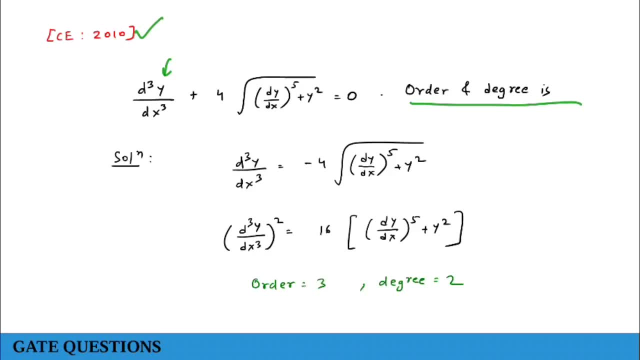 okay, where is the maximum of n? maximum of n is here, so n is equal to 3. is our order correct? and what is the power? power is 1, so degree would be 1.. so this is wrong. this is completely wrong, because i have told you: if you have this radical, this fraction, if you have this fraction, get rid. 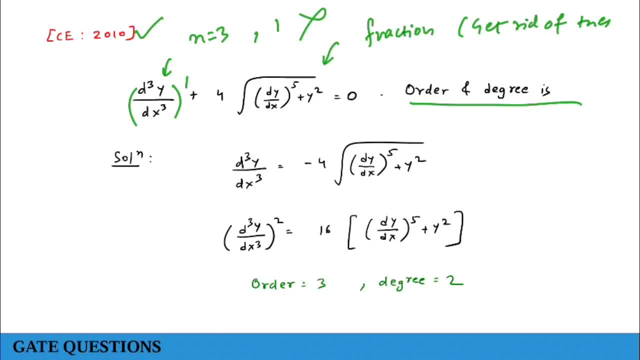 get rid of this fraction. so how to get rid of this fraction? because if you do the square square part, it would be a big mess. so what you can do is you can rearrange, rearrange this equation. what i have done is i took the, i took this function, i put that in the right. 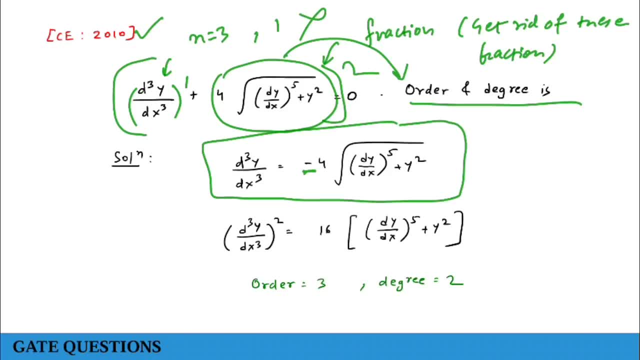 inside. so now i will get minus sign correct because this function has gone to the right inside. now you can see i can do square on both the side. it won't be a mess. so if i do square on both the side, this term would be the whole square and here the radical would be eliminated. so this radical has eliminated. 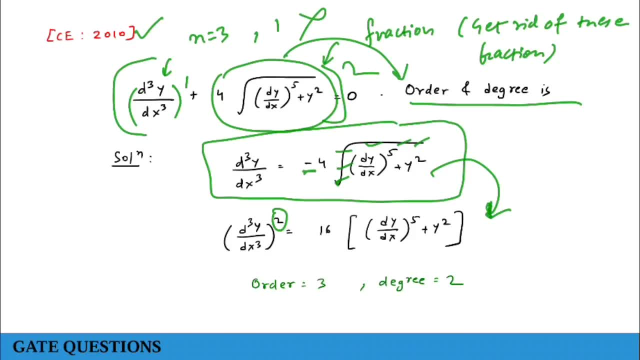 the whole square. so now you have to ask yourself what is the maximum of n? here n is equal to 2. here n is equal to 1, so n is equal to 3 is maximum. n is equal to 3, so our order is 3. and what is the?